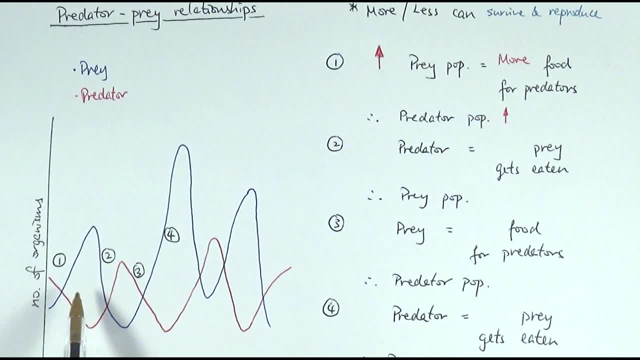 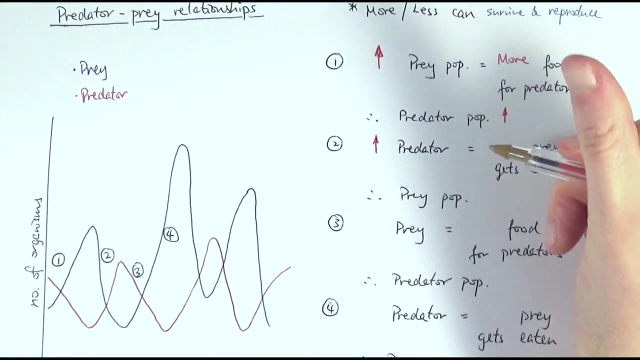 would increase after some time. So as it goes up, then this one also, the predator curve also goes up eventually, And as the predator population increases. so that's kind of following up on the next point, stage two: so as the predator population increases, more prey would then get, will be. 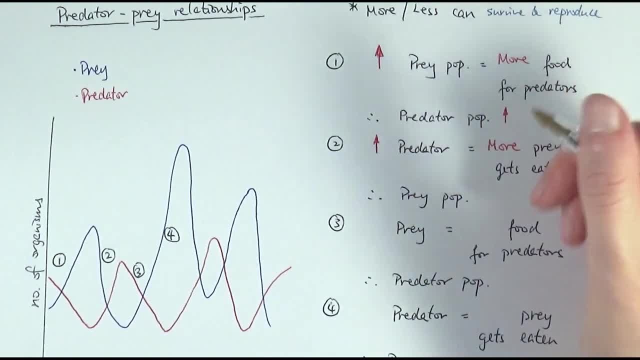 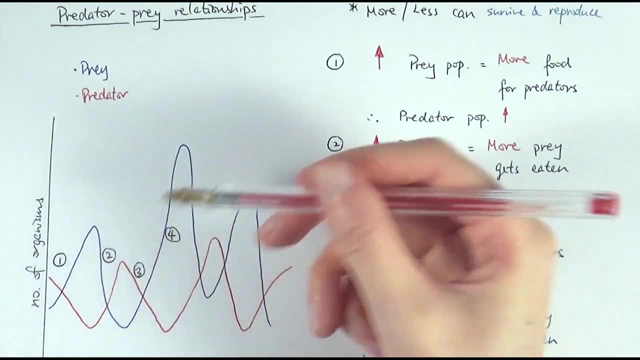 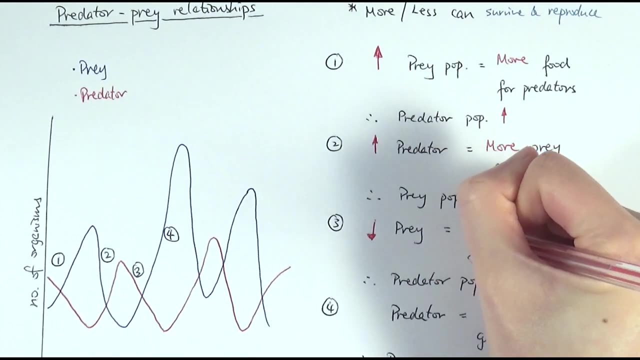 eaten, So therefore less prey can survive And produce. therefore the prey population would decrease. So, as you can see in the graph, the prey population decreases as the predator population increase there. And then the third stage: as there is less prey available, that means less food available. 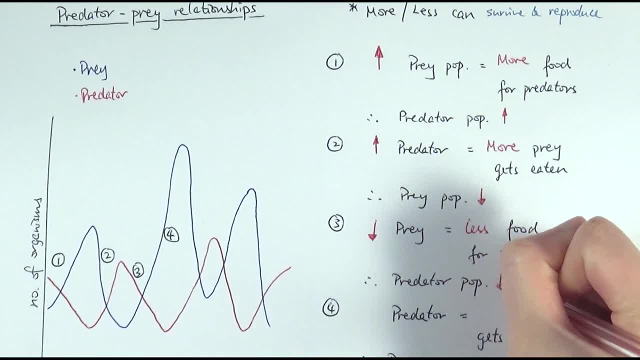 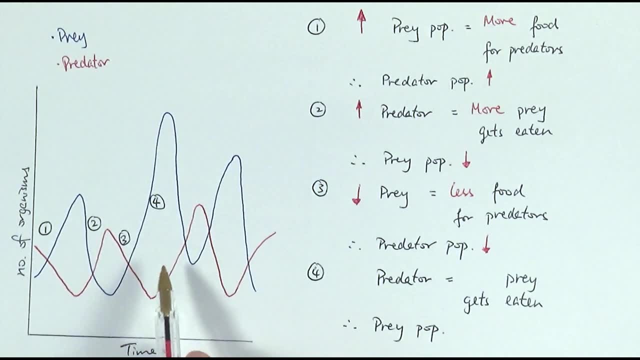 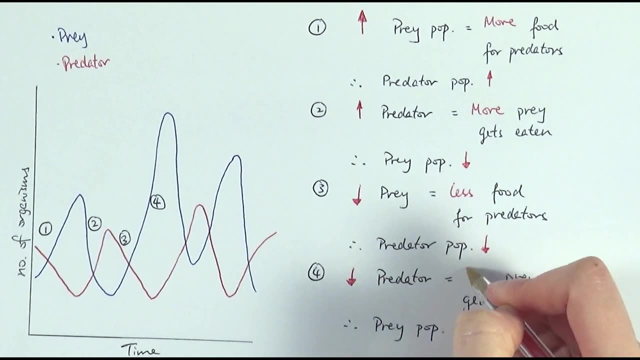 for the predators. therefore, the predator population would decrease as well, because less predator can survive and produce due to the loss of food source. And then, finally, the last point, because there is less. There are less predators there hunting them, so therefore less prey gets eaten. therefore, 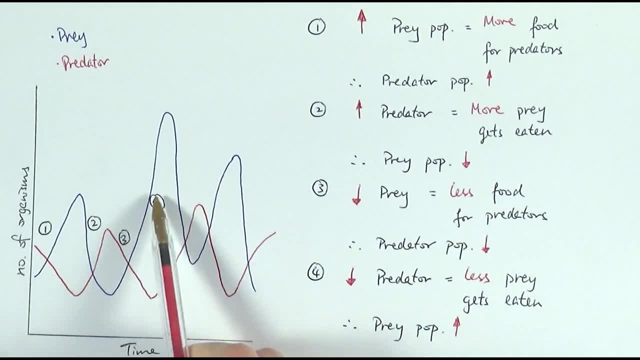 the prey population would increase once more, as shown in stage four. As prey predator population decrease, less prey gets eaten, the prey population can increase massively again. So, as you can see, the population sizes of the prey and the predator follow each other. 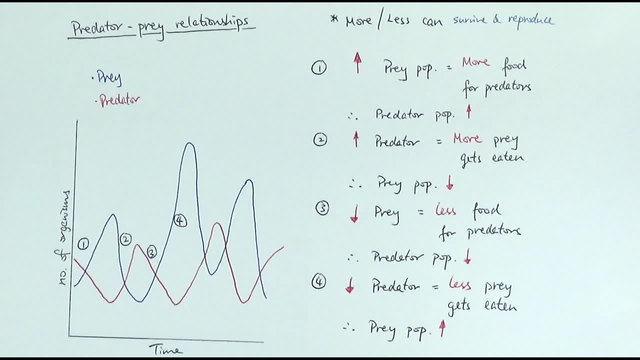 They show the same trend and the same pattern, And that is the predator and prey relationship. Thank you 1. 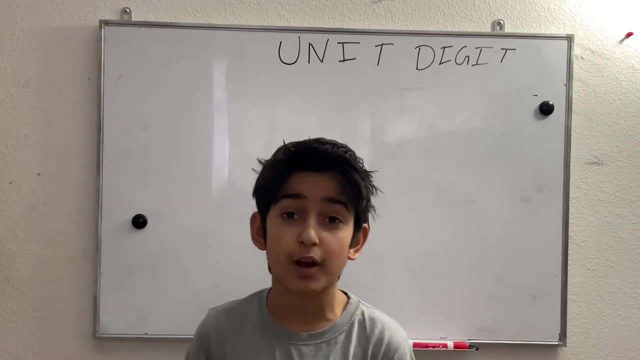 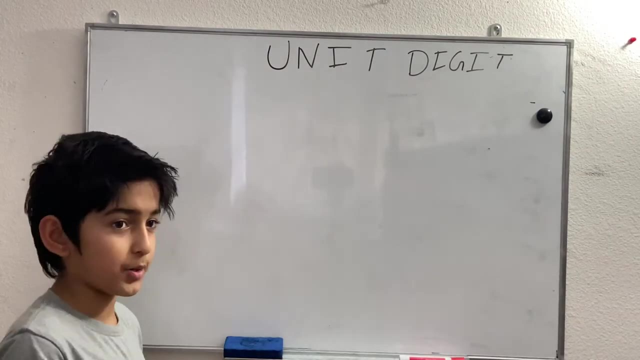 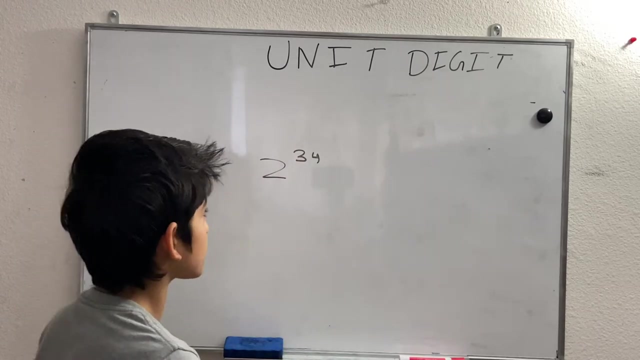 Hey guys and welcome to Learning Math. Today I'll be going over how to find the unit digit of an exponent. So let's get into it. So let's find out the unit digit of an exponent. So here's an example of two's power, let's say 34.. Okay, the first thing you have to do is write. 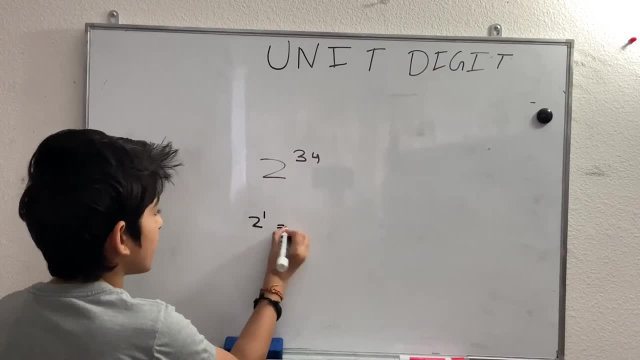 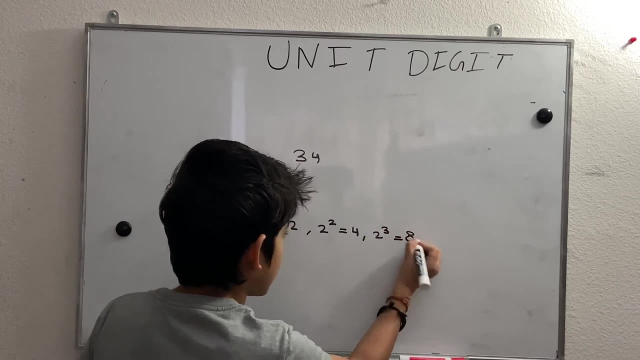 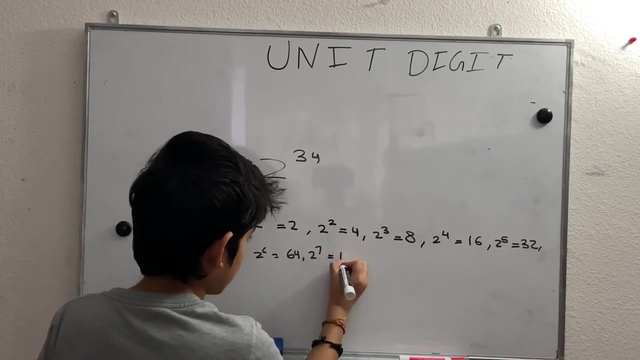 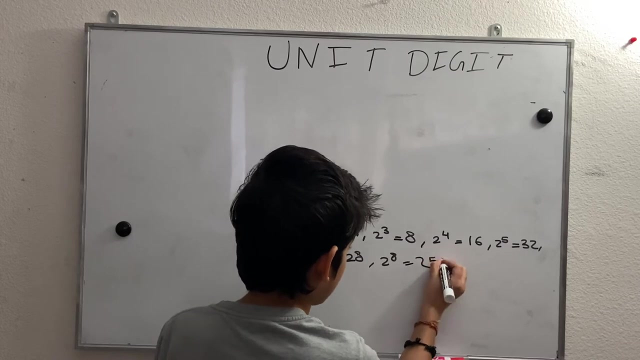 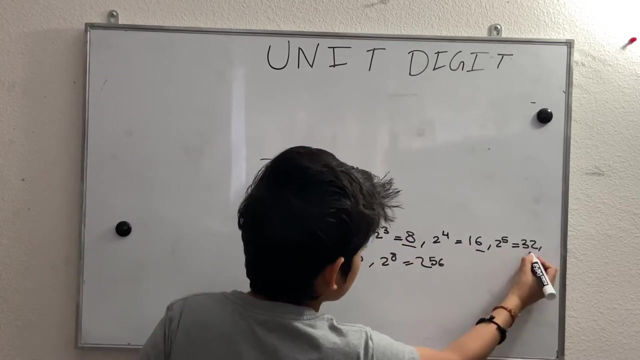 two's power until about eight. let's say: Two's power one is two. two's power two is four. two's power three is eight. two's power seven is 128, finally, two's power eight is 256.. Now underline the unit's digit, as I just said. So two, four, eight, six. two, four, eight six.